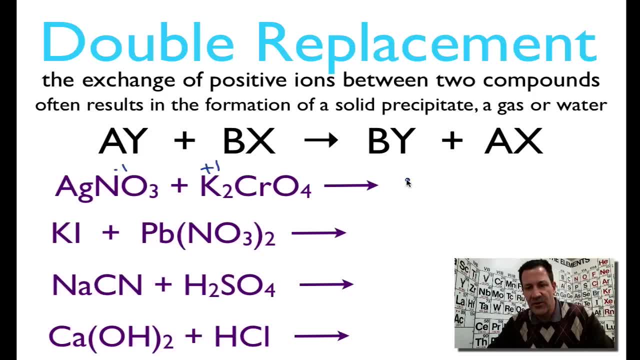 plus one nitrate is minus one. so we know that we're going to have one to one, potassium and nitrate to form, obviously, Our potassium nitrate, KNO3. that is supposed to be three, Alright, and plus we're going to have silver chromate. Well, silver forms plus one charge. 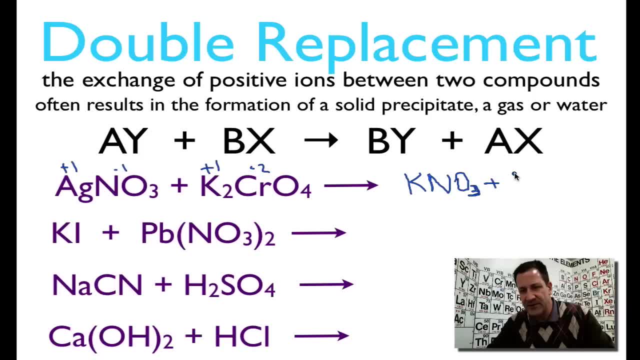 chromate forms a minus two charge. so that tells us that this is going to be Ag2CrO4.. Okay, so silver nitrate plus potassium chromate will form potassium nitrate and silver chromate, and let's see if we can balance that. We have two potassiums over here. 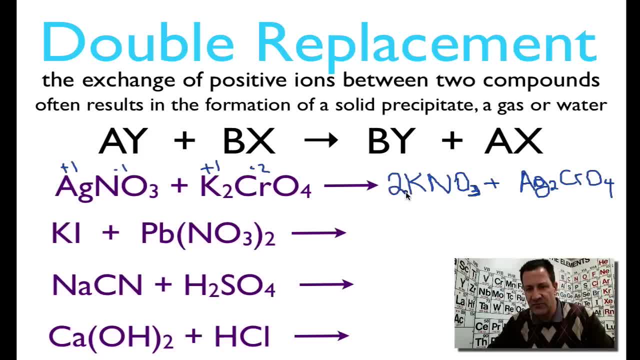 which tells us we're going to have to have two potassiums over here and that tells us we're going to have two nitrates. We have to put two here in front of the silver and let's say we have two silvers and two silvers and one chromate and one. 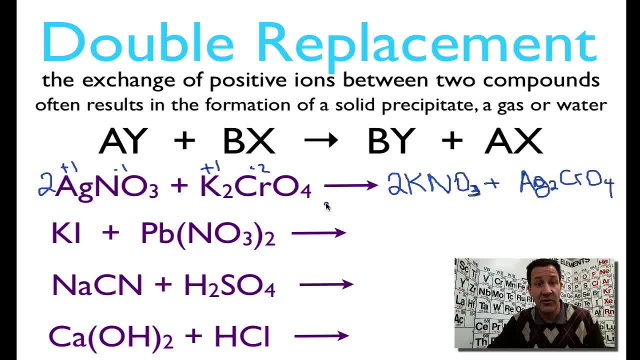 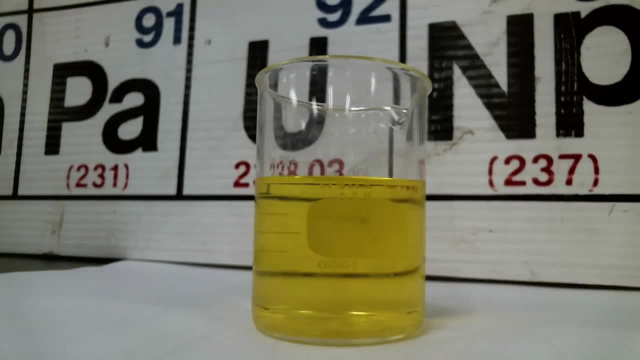 chromate. Okay, so that is the double replacement reaction for potassium chromate. Now, before we go on to the next one, I am going to show you this double replacement reaction. So let's go do that Right now. Okay, so now I'm going to perform the double displacement reaction. 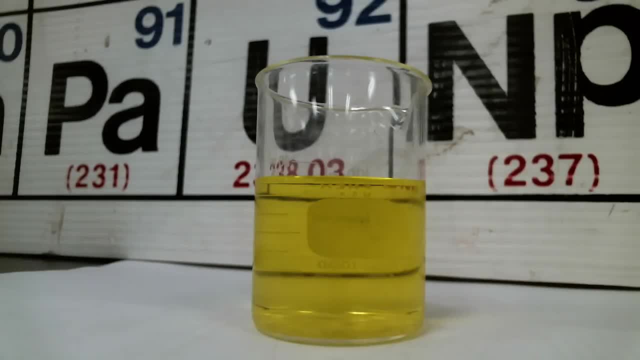 between silver nitrate and potassium chromate. and here you can see, I have my solution. I have an aqueous solution of potassium chromate and I'm going to add to that from my pipette. I'm going to add some silver nitrate. I'm just going to 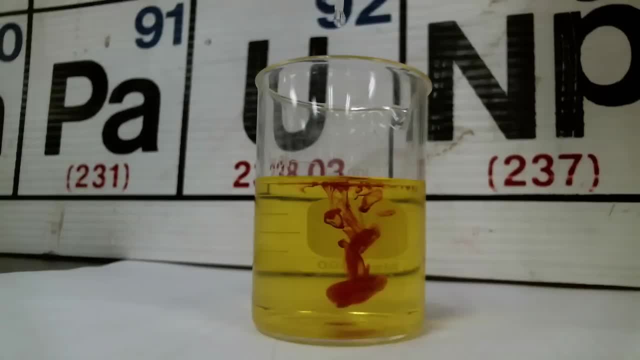 drop a few drops in here and you can see that very nicely. it forms a very pretty brown red precipitate and that is the double displacement reaction. That is the result of the double replacement reaction between those two compounds. It's actually solid. It doesn't really look like a solid, but if I pass it through a 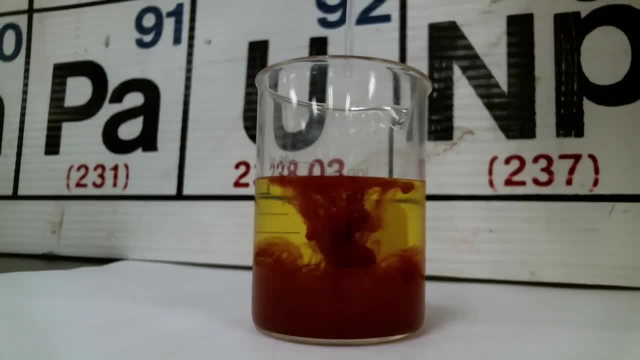 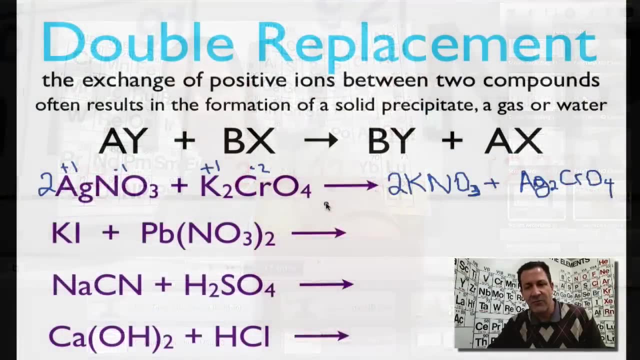 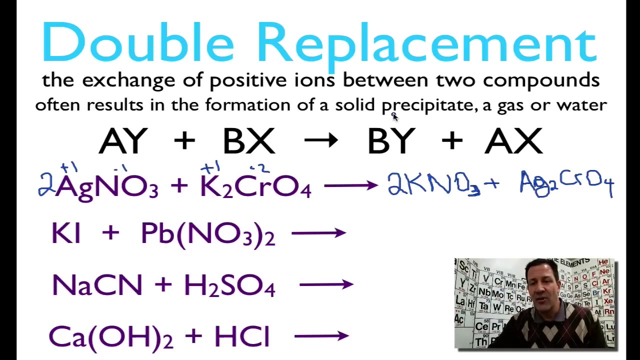 filter, I can filter it out, and that is the reaction between potassium chromate and silver nitrate. Okay, that worked out really well. We formed that reddish brown solid. Oftentimes it forms a precipitate and let's see if we can figure out what. 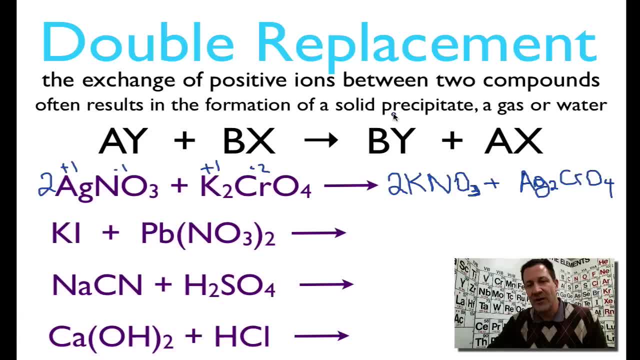 that reddish brown solid is. In order to do that, we're going to have to now turn to our solubility table. So let's get our solubility table out and look and see if we can figure out on our solubility table what that reddish brown solid is. 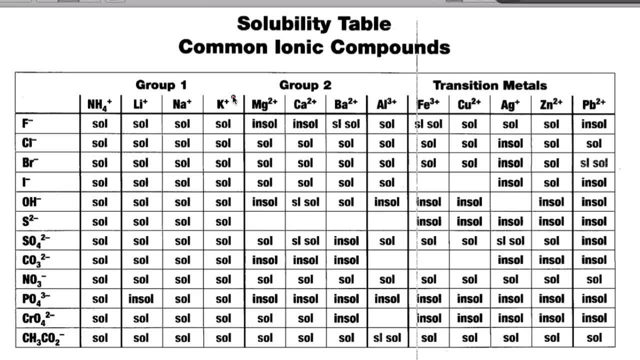 Okay, so here you can see, we have our solubility table. We have our positive ions on the top and our negative ions and our polyatomic ions on the left hand side, and we want to see which of those two, the potassium nitrate or the silver. 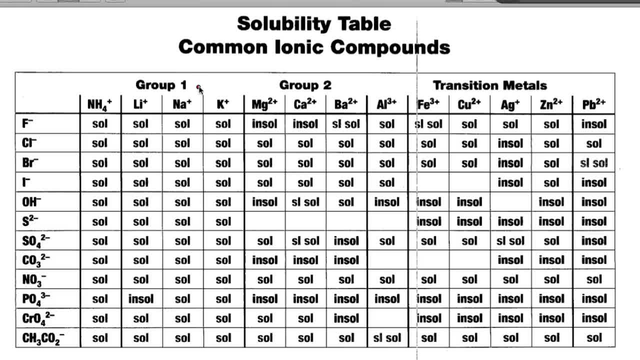 chromate of our products is that insoluble solid. So let's just look at the first one which we have: potassium is here And we have nitrate is over here And you can see, if we follow nitrate over and potassium down, we come to this square right here and it says SOL and that. 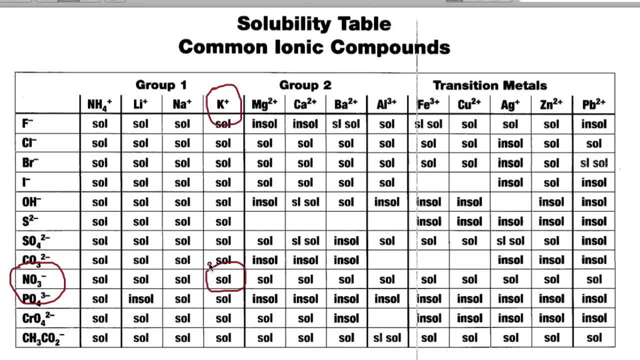 means that that is soluble. So that is not the solid that we produced. And let's see. the next one was silver and chromate. So here is chromate and over here is silver, And you can see if we follow the silver and the chromate. 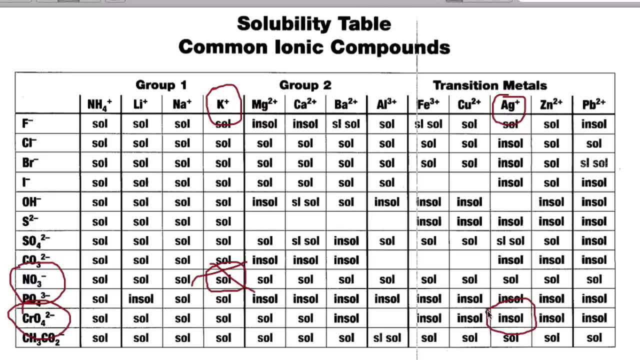 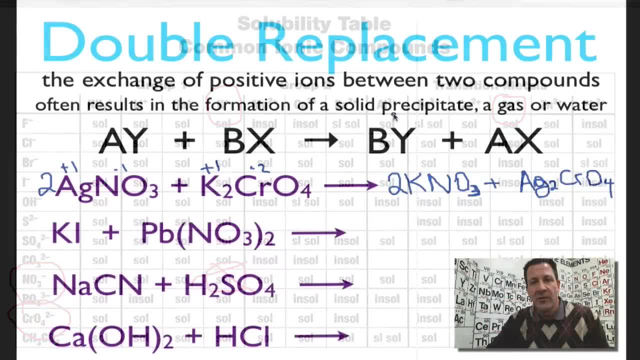 that they intersect right here And that says insoluble, and that tells us that, yes, indeed, that solid, that precipitate, that red-brown precipitate that we formed, is actually silver chromate. Alright, so let's go back and do another one. Okay, that's right, that was silver chromate, That was our insoluble compound. 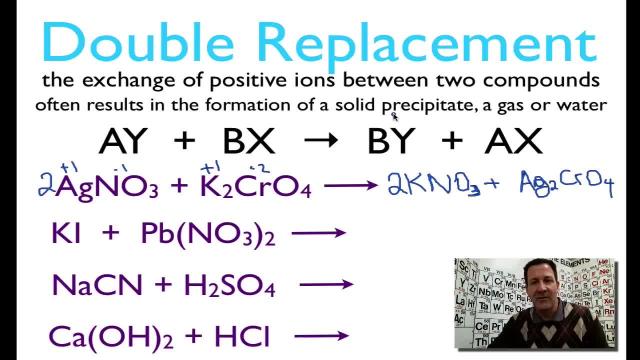 the potassium nitrate being soluble. Okay, now let's go through and let's do the next one, This one: we have potassium iodide and then we have, yeah, potassium iodide and lead nitrate, And in this case, we know, let's do the. 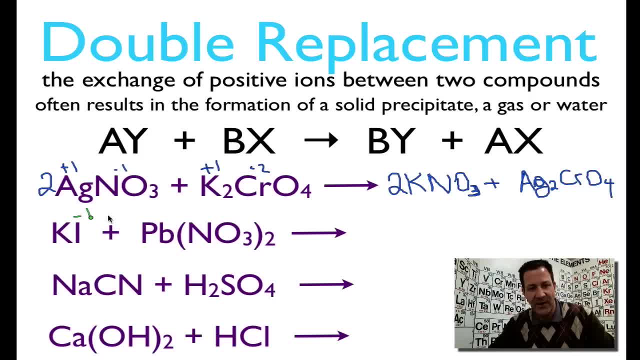 inner two. first, We know that potassium forms, excuse me, the iodide forms- a minus one. Lead is plus two. So we know that in this equation, one of our reactants or one of our products, excuse me, it's going to be PbI2.. And then the other product is the. 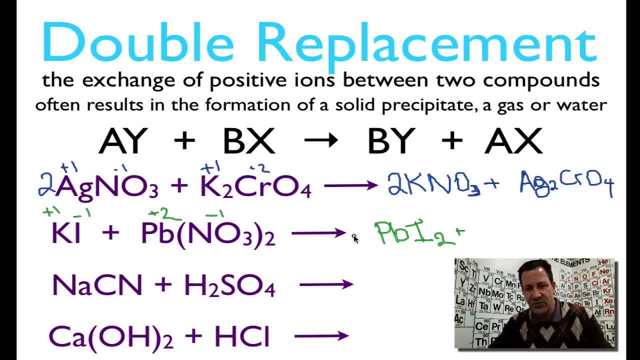 potassium, which is plus one, the nitrate, which is minus one, and once again, in this one we're going to have K2., NO3. And let's balance that. We have two iodines, So we're going to have to put a. 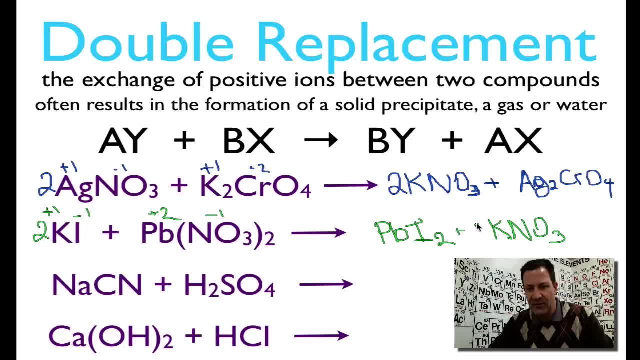 two here, two potassiums. We're going to have to put a two there. I think that's balanced, because two potassiums, two nitrates, two potassiums, two iodines, two nitrates and one lead. Okay, so that's balanced like that, And once again, I'm going to show you this. 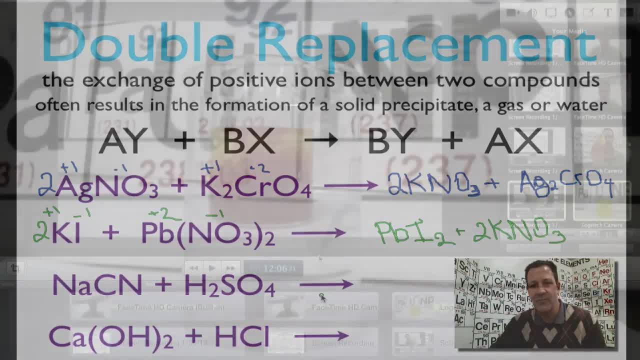 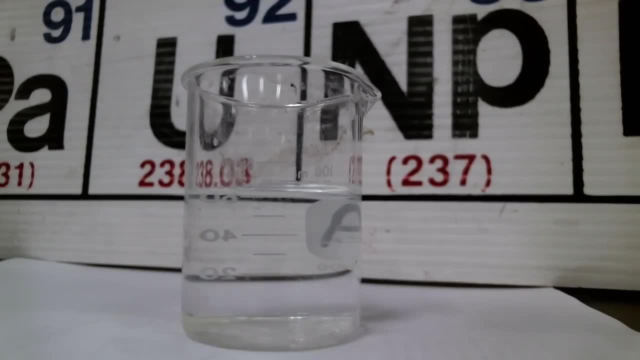 double replacement reaction. So let's go and do that reaction right now. Okay, now we're going to do the double displacement reaction between lead nitrate and potassium iodide, And you can see in my beaker, here I have my solution of lead nitrate and then from 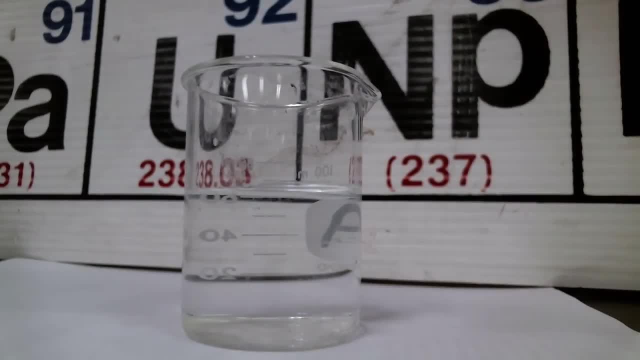 my pipette. I'm going to add some potassium iodide. I'm just going to put a few drops in here at a time and we'll see what we get out of that reaction. You can see, we get that very beautiful canary yellow color. That's a solid, That's a 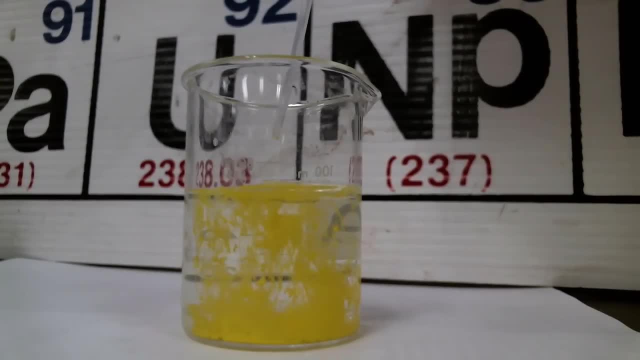 precipitate. It might not look like a solid but it's in solution, and if we wanted to get past that through a filter and then we could get from that the solid onto the filter. So that is the solid that is the result of the reaction between potassium iodide. 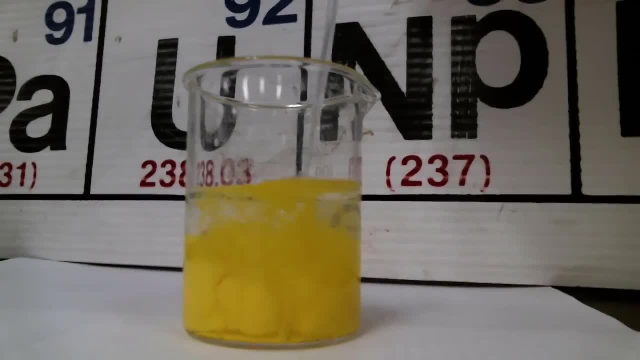 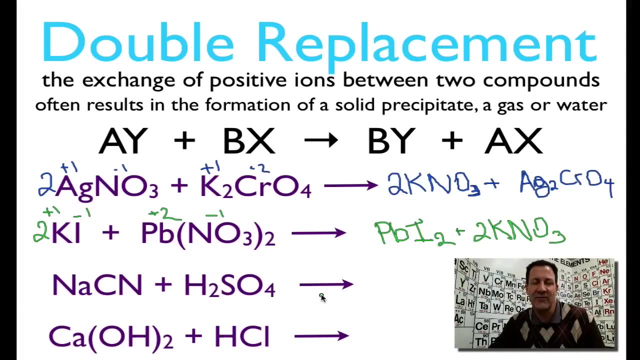 and lead nitrate. Okay, that's a very beautiful reaction. I like that. Double replacement reactions don't tend to be very flashy, but they are very beautiful. You have that solid formed, That's that yellow solid, And let's see if we can figure out, using our solubility table, what that yellow 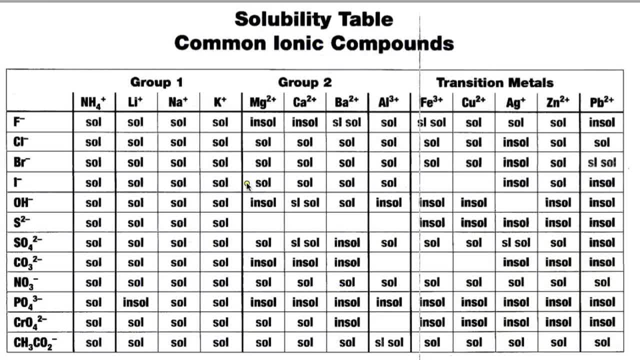 solid is Okay. so here is our solubility table again. And we know from the previous reaction we formed. in this reaction also we formed potassium nitrate And we know from the previous reaction that that is soluble. So that yellow stuff is not potassium nitrate, because that is a soluble compound. Now 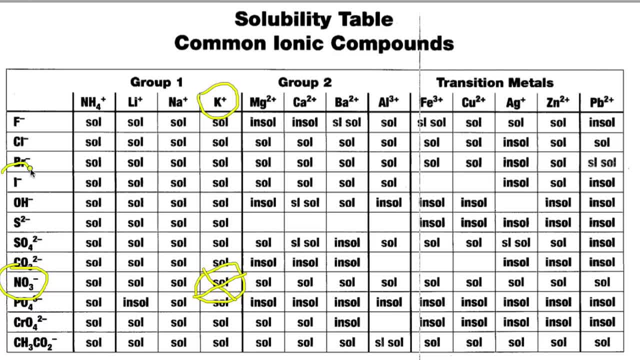 let's look at the other compound that we formed. The other product was lead iodide. So there's the iodide and here is the lead. So we fold the lead over and the iodide down. We see that here it is. We see that that is insoluble. So that yellow solid, that precipitate, that we 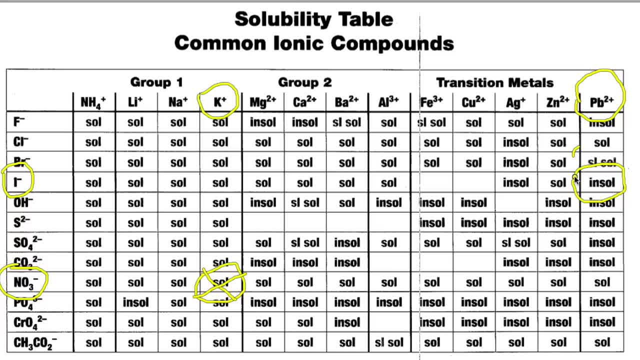 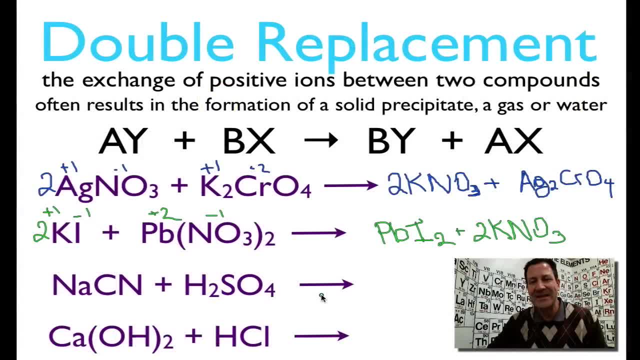 formed in that case was PbI2, which is lead iodide. All right, Very good, Let's go back and do another reaction. Okay, so that's right, That yellow solid is lead iodide. That nice yellow canary yellow solid. 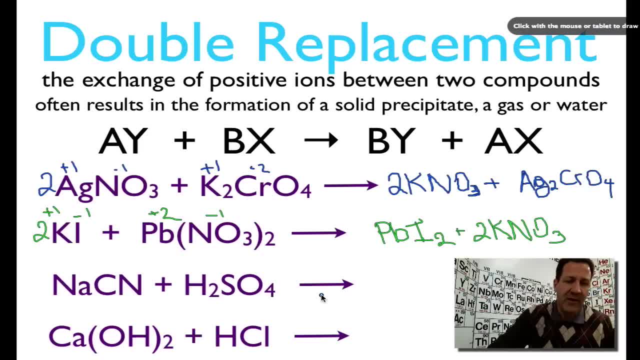 Okay, let's go and do the next one. This time we have sodium, cyanide and sulfuric acid. We have one, two, three, four different things. We're going to recombine them. Let's do the sodium and the sulfate first. Sodium forms a plus one charge. 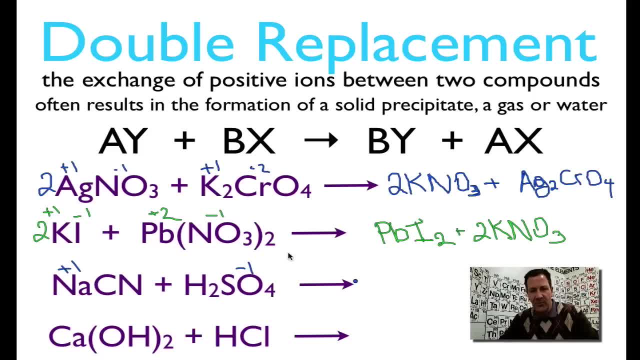 Sulfur is minus one, So we know that's not true. Sulfate is minus two, So we know that one of our products is going to be Na. We need two sodiums to satisfy one minus two sulfate. And then that the 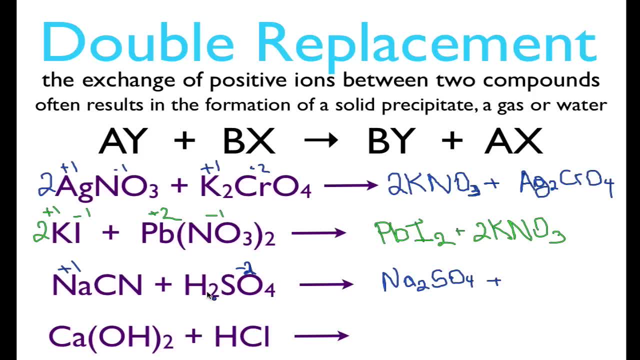 other product is going to be hydrogen cyanide, And hydrogen is obviously plus one And cyanide, if you don't know, is minus one. So that is going to be hydrogen cyanide And let's see what we need to balance. We have two hydrogens, two 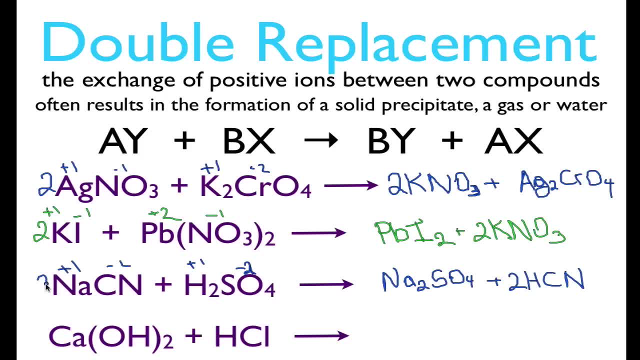 hydrogens, two cyanides- we need two over here- And that satisfies our two sodiums and our one sulfate, and that chemical equation is balanced, just like that. Ok, One more, Oh, and then this is a gas. Hydrogen cyanide is a gas, So we have a. 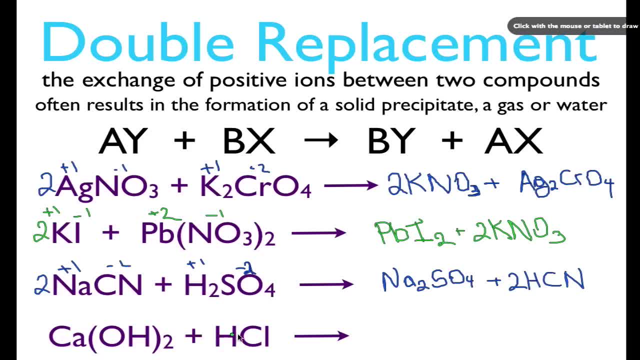 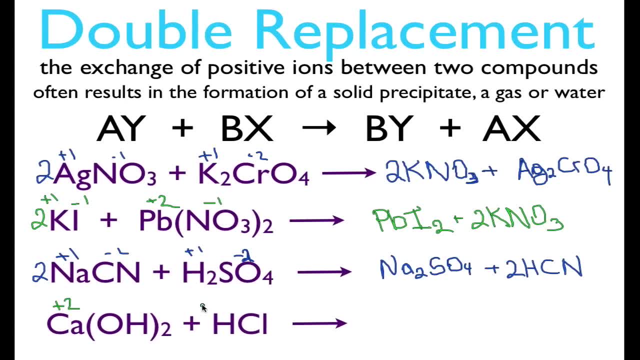 gas being formed in this one. So now we have calcium hydroxide and hydrochloric acids. So we have one, two, three, four ions here, and calcium is plus two, chlorine is minus one. so when we have our potassium chloride, when we consume our calcium chloride, we recombine our outer elements. it's 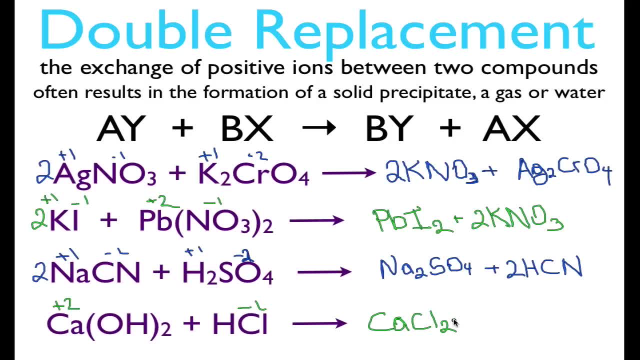 CaCl2, and then the other one is going to be the hydroxide and the hydrogen, and sometimes you see it written as HOH, but that's just a plus sign here, HOH, and we can just write that because we have two hydrogens and an oxygen, and that, of course, is H2O, which is water. so that reaction. 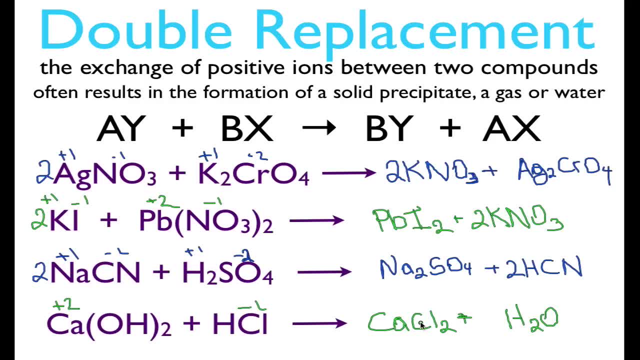 produces water. Okay, now let's see. we need a balance. we have two chlorines and that tells us we're going to have to put a two here, which gives us two hydrogens. we have two hydrogens and let's. 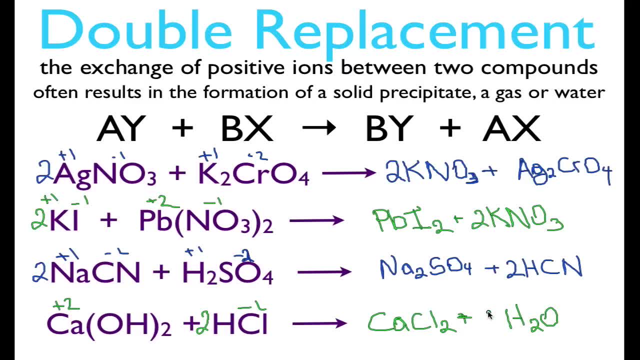 see we actually have on this side. we have two here and two here. that's four. so we're going to need two more here for two hydrogens and that gives us two oxygens. we have two oxygens, one calcium one. 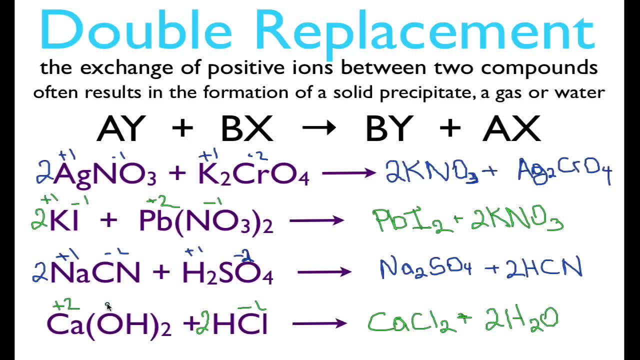 calcium. Okay, so there you go. that chemical equation is balanced, and we want to just maybe put them together, Minus one and plus one, since we're trying to be complete here. All right, so that takes care of all of that. We have our double replacement reactions. we have two compounds, four ions on the left and 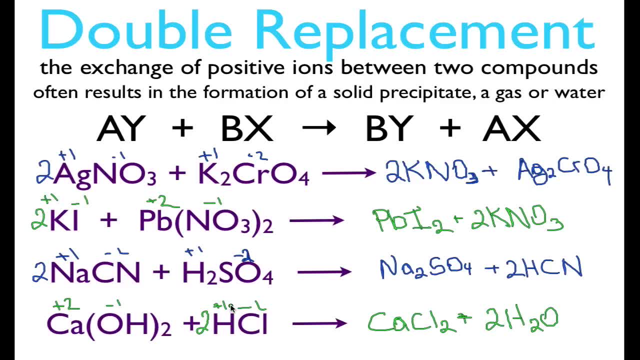 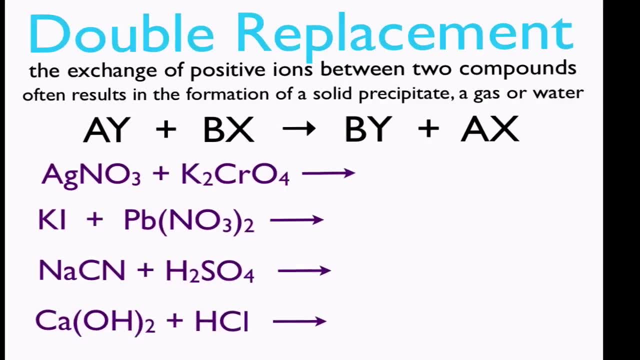 two compounds and four ions on the right, and that is how you can identify a double replacement reaction. Okay, so, thank you very much. thanks for watching. I hope that was helpful and we will see you next time.